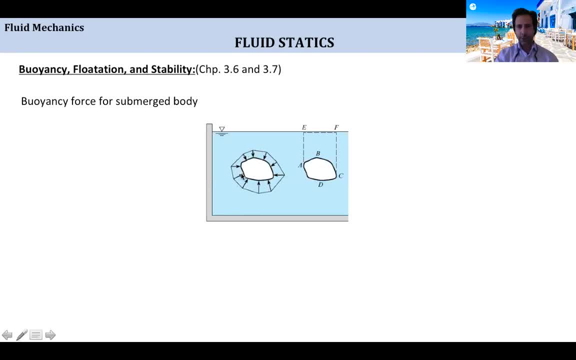 as depth increases, pressure forces increase And you can see this increase from the length of these pressure force vectors. Now you can follow a similar procedure that we considered for the pressure force on curved surfaces in the previous module. This is also explained in your textbook And you can show that this. 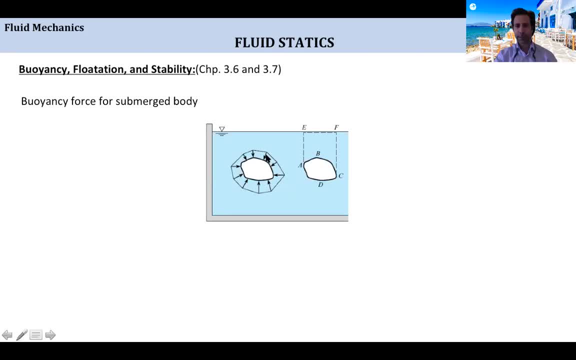 force distribution will result in a net vertical pressure force And if you look at this schematic, you can see that horizontal components of these forces cancel each other and vertical forces are unbalanced. We have smaller vertical forces which are unbalanced and we have smaller vertical forces which are. 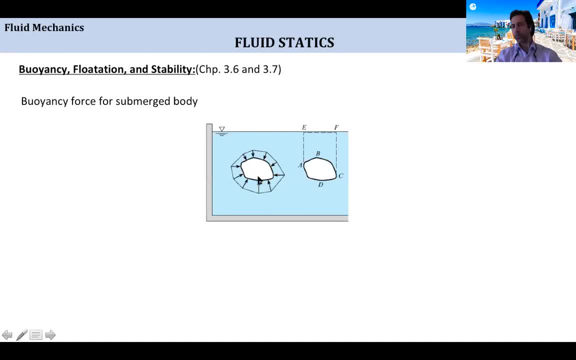 unbalanced. We have smaller vertical forces which are unbalanced. We have smaller vertical forces acting downward than vertical forces, you know, acting upward. so, as a result, we have a net vertical upward force and this is the buoyancy force, and we will- first we will consider two types of objects. one is for buoyancy forces, on 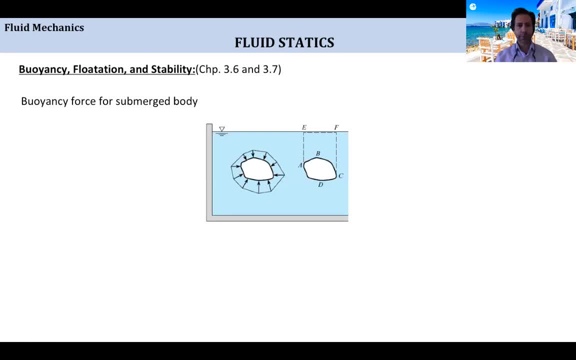 submerged objects and also we will consider buoyancy forces on floating objects. when I say submerged body, it may be stationary within the fluid column, so there may be some sort of an equilibrium and the object is floating within the body. well, let me rephrase: it's submerged within the fluid and it is. 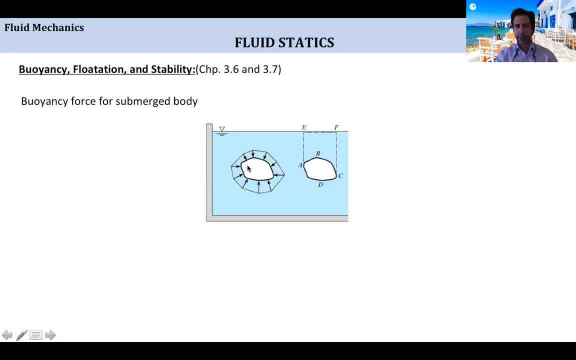 somewhere within the fluid column, as you can see here, or it may sink all the way down to the bottom, and it is still a submerged body, or- and we will also consider the floating objects- which the object is partially submerged and partially, you know, above the fluid surface. now let's first consider the buoyancy force, for 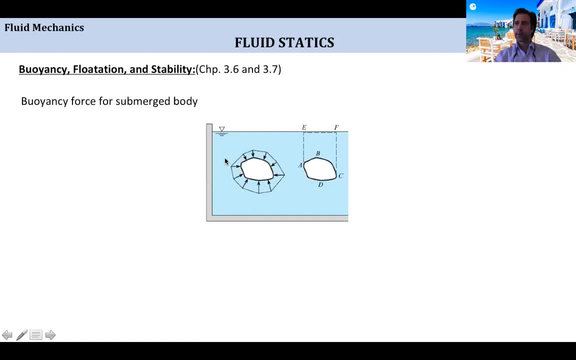 submerged bodies. but before that I want to read couple of important remarks for the buoyancy and floatation and I will read them so that I don't confuse you these statements. so we have two important remarks about buoyancy and floatation concepts. the first one is we say that a body 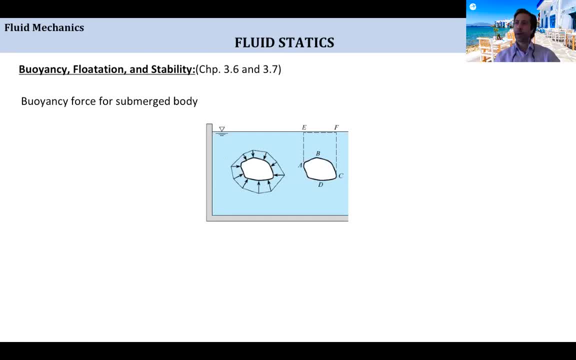 immersed in a fluid is buoyed up by a force equal to the weight of the fluid displaced. okay, so I'm repeating again: a body immersed in a fluid is buoyed up by a force equal to the weight of the fluid displaced, and we will mathematically represent this expression very soon and the 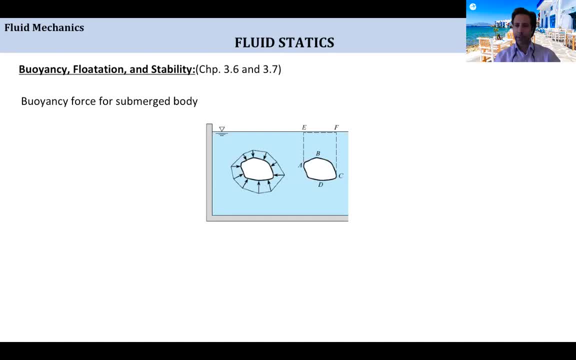 second important remark is: a floating body displaces its own weight of the liquid in which it floats. okay, i'm reading this second remark again: a floating body displaces its own weight of the liquid in which it floats. okay, so these are two important remarks and starting points for our 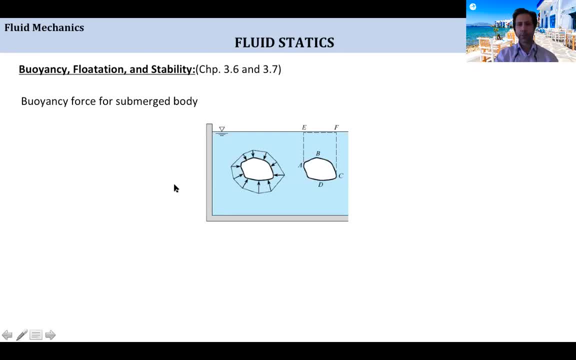 next discussion. so for the buoyancy force, for submerged body, buoyancy force can be calculated as specific weight of the liquid. so whatever the liquid is- it may be water, it may be oil- so specific weight of the liquid multiplied by the volume of the object. so this is the body, so volume of the this body, or volume of 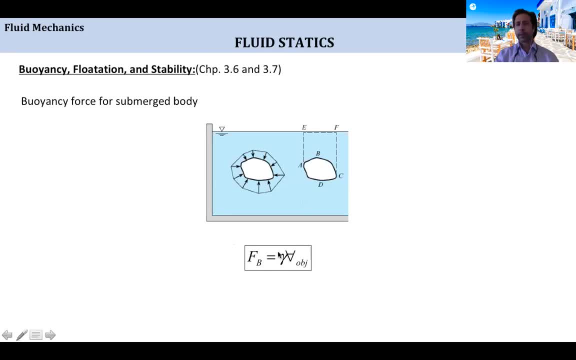 this object. now, this is remember. our first remark was: a body immersed in a fluid is buoyed up by a force equal to the weight of the fluid displaced. so this is the volume of the object. so this is the volume of the object. so this is the volume of the. 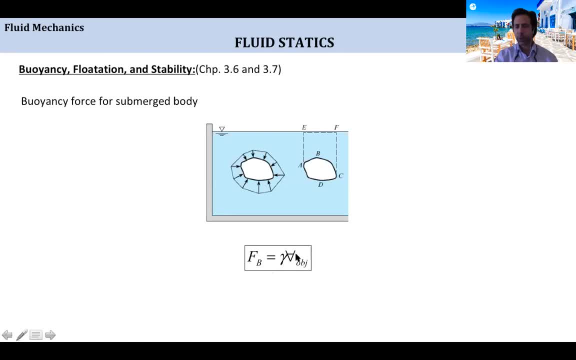 liquid". so first we estimate the volume of the liquid and then- this is our next moment- how that volume of the liquid would explain anything we know, and that then we analyze as what, ah, where do we find aided that was taken over from the liquid anyways. so basically, this is the action of the equation. so the x entrev dre can regre conversation. 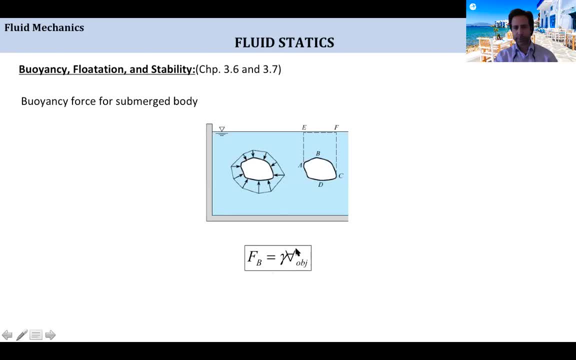 Programming, there's a volume of the fluid and the volume of the object. all we do is list the volume of a thing as if this was it wirklich there, all weAs, so all nude across this range. so these prepared all values have been dropped. lead is from ground to the liquid, and so can check them all in order to see if there is a result. and now we can взt Wenn bless muut das ohne Sie Linz. 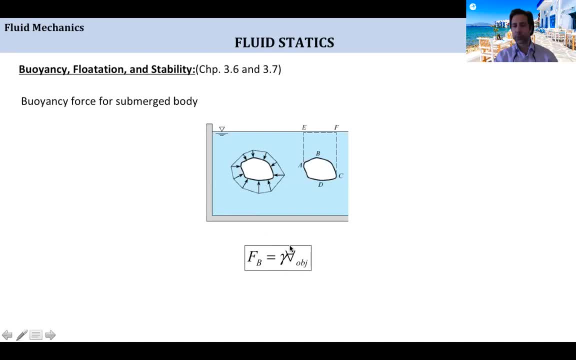 we would get the weight of the fluid that is displaced by this submerged object. so this is how we calculate the buoyancy force for the submerged object. now the second type of objects that we will consider is floating objects. now for the buoyancy force for the floating objects. here you can see that this is the volume displaced. this is the volume of the fluid. 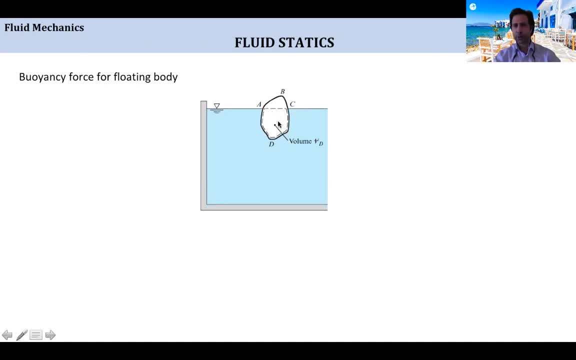 displaced by the object. this is the submerged part of the floating object, right? so this is the dashed volume. is the volume, uh, displaced now? so the buoyancy force will be equal to specific weight of the fluid multiplied by the volume displaced. right. volume displaced, so which is this dashed volume? so this would be the weight of the fluid. 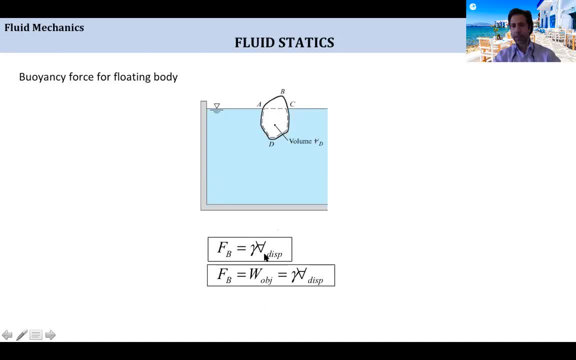 displaced. right now, this floating object is at a static equilibrium position. it is not sinking, so it is resting at the fluid surface, which means that weight of the fluid, the object, is compounded, or uh, so weight of the object is equal to the uh, the buoyancy force created by the fluid. otherwise, 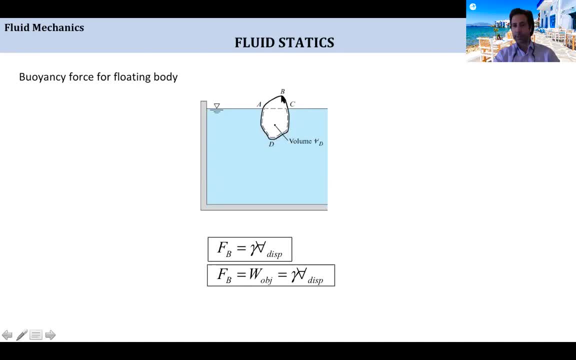 if the buoyancy force would be, it was less than the object would sink right, so it would be submerged. but since this is at a stationary- you know it's, it's at a static equilibrium, we can say that summation of the force in the vertical direction is equal to that force in the balance direction. 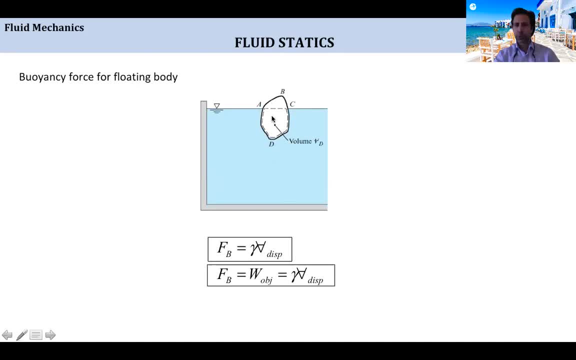 are equal and we know that one of the forces is buoyancy force, which is vertical up, and the other force is weight force, which is vertical down, and since there is equilibrium, weight should be equal to the buoyancy force. so we can say that buoyancy force is equal to weight of the object, which is 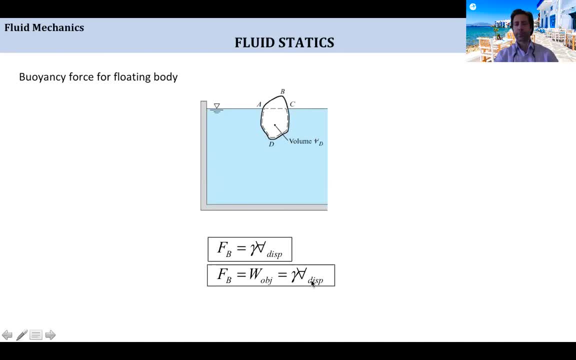 equal to specific weight times, volume displaced. to make things easier, we can express these, the two remarks that i have provided earlier, with this one mathematical formulation. so basically we can say that buoyancy force is specific weight of the liquid multiplied by the volume displaced. if it was a submerged object, then volume displaced is: 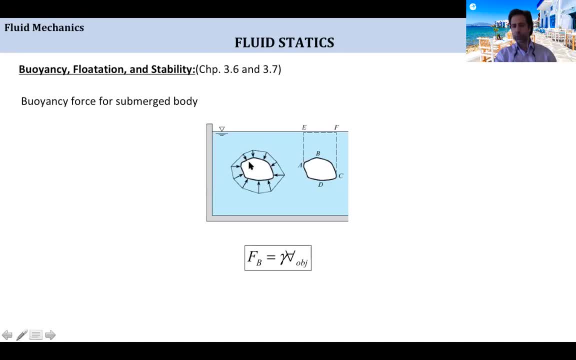 equal to the volume of the object because it's completely submerged. so this equation is applicable for both the submerged and floating objects. you just need to consider that volume displaced is equal to volume of the object when it is completely submerged and when it is floating you just need to consider the submerged portion of the volume to calculate. 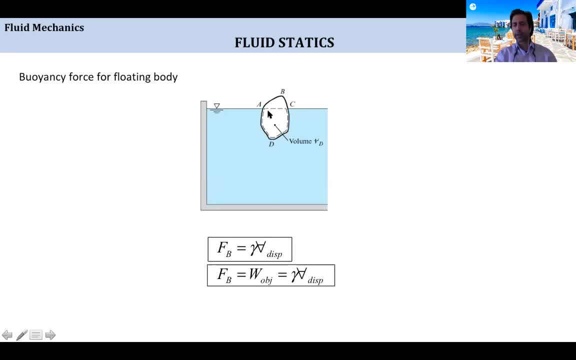 the volume displaced and when it is floating. we know that, as we discussed, weight should be equal to the buoyancy force, so we can use this condition for the static equilibrium condition. now, this buoyancy concept, this buoyancy force, is what we use to float, for example, ships. 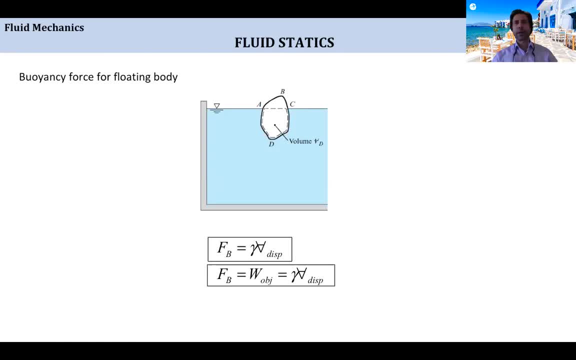 right. so if you consider, modern ships are made of heavier materials, let's say steel or some you know metal alloys, etc. so these materials have higher density than the liquid itself, which is water or sea water, right. but despite this density difference, these ships can float and travel over the you know sea. and the reason is: 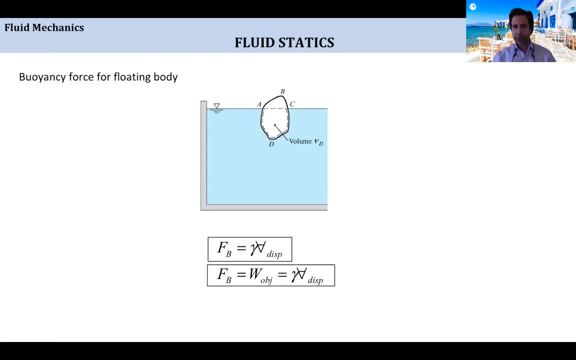 we shape. we shape these objects, these material okay to form objects that displaces sufficient amount of water that would be equal to the weight of the object. so this is where the design comes into play. so we can shape a metal and we can have it swim or float over a liquid surface with proper design. this is what we do for concrete canoes also, okay. 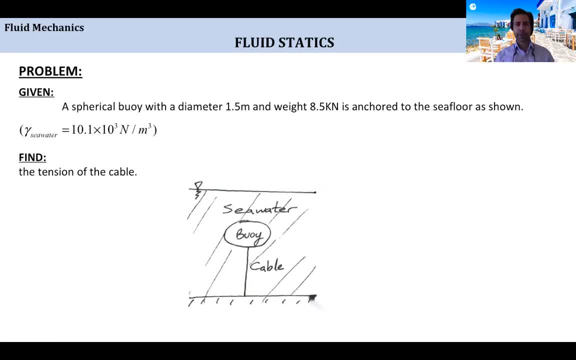 now let's solve an example problem to demonstrate these concepts. so in this problem we have a spherical buoy. you can see here this buoy is anchored to the sea floor through a cable and this is, let's say, in a coastal zone or an estuary or so. so let's say we have sea water. 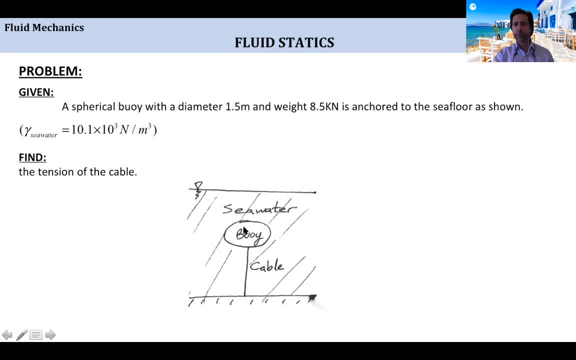 and the buoy has a diameter of 1.5 meters. it has a weight of 8.5 kilos newton and we are given that a specific weight of sea water is 10.1 times 10 to the 3 newton per. 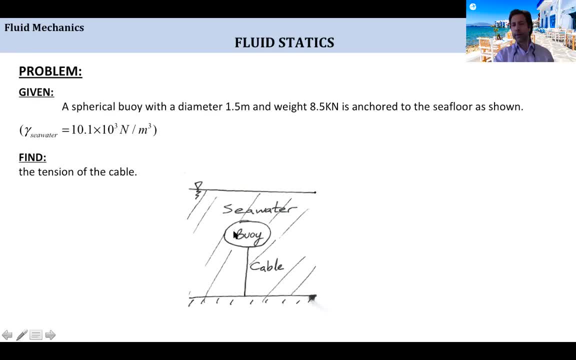 meter cube. typically these buoys are, to you know, float over the surface and they are typically instrumented or perhaps some other purposes. but sometimes water level changes, such as for example during times of tides, and as a result that buoy may be submerged. so we are asked to find the tension of the cable when it is submerged. 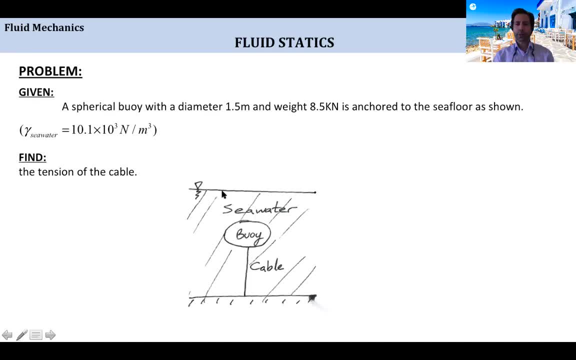 as you can see here in the schematic. and of course, when we are designing such a system, such a buoy or such an- you know- attachment, we need to consider forces, a range of forces that the cable and the anchoring can resist, so that buoy is not damaged during different. 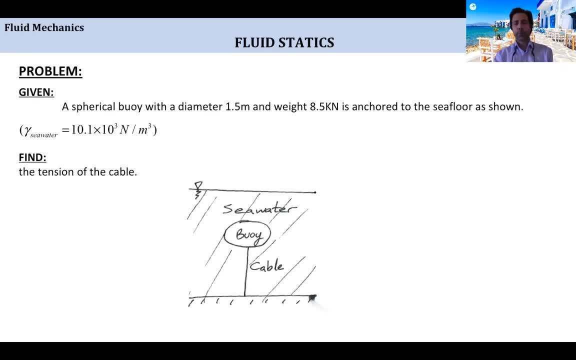 environmental conditions. so i would recommend you to pause the video here and try to solve this problem on your own and then restart the video and compare your solution with the solution that we will go over next. all right, so here i kept the uh problem schematic uh on the right for your convenience. 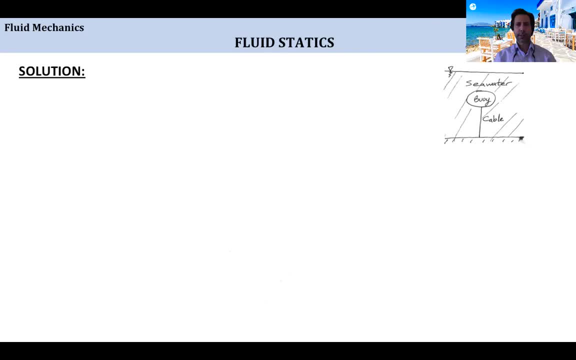 the first thing we need to do is we need to consider the forces acting on this object, which means that we will draw the free body diagram. so, if you consider the free body diagram, this is the spherical buoy we have, and we have buoyancy force acting on this buoy, which is vertical up. 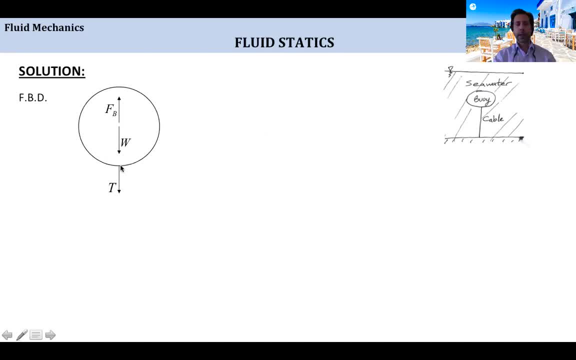 of the buoy, which is vertical down, and we have also tension force due to the cable. so cable is pulling the buoy down, so we have a tension force acting downward. so this is these are the three forces acting on the buoy. now we know that there should be a static equilibrium for a stationary 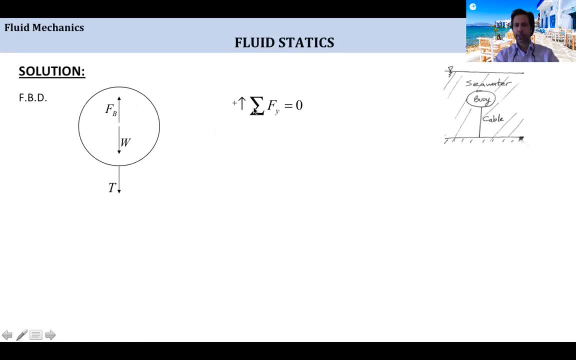 buoy we, which means that vertical force is acting on the buoy in y direction right should be equal to zero. if we consider positive y direction as vertical up, then we can. our equation, the equilibrium equation in y direction, states that buoyancy force minus weight, minus tension, equals to zero. so from here tension is equal to buoyancy. 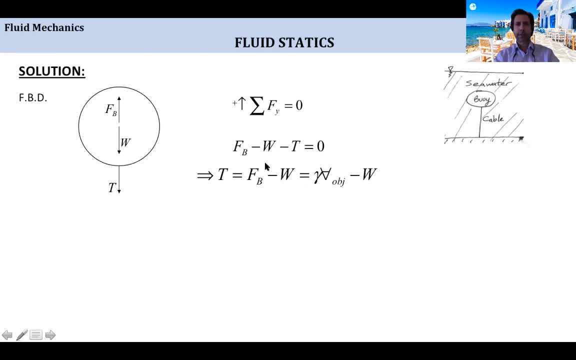 force minus weight. and it says we know that buoyancy force is the specific weight of the fluid times. volume of the object. it's a submerged object, so we consider volume of the object which is equal to volume displaced. so we consider volume of the object minus weight. 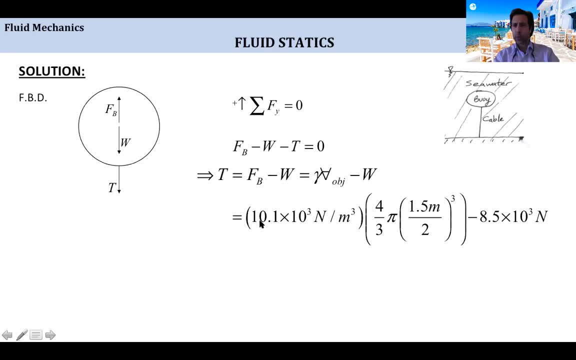 now in the problem we it's given that the specific weight of the seawater is given as temperature, 0.1 times 10 to the 3 newton per meter cube. we know that's the spherical buoy. so volume of the object can be calculated as 4 over 3 pi. the radius is given as sorry. diameter is given as 1.5 meters. 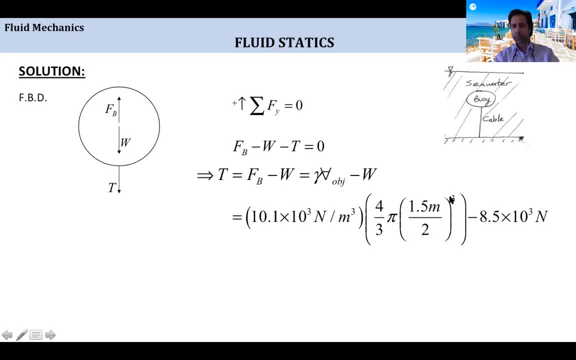 in this problem. so radius is 1.5 over 2 and we take the cube of it to calculate volume of the sphere. then we also know that the weight of the buoy is 8.5 kilo newtons, which is 8.5 times 10 to the 3 newtons. so if we do the calculations we can show. 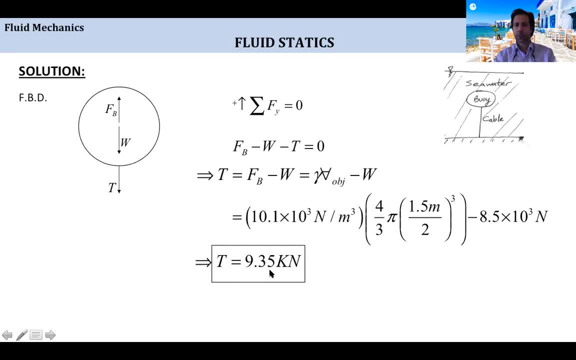 that the tension force acting on the buoy is 9.35 kilo newtons. now, this is the answer to our problem. next we will discuss the stability of submerged and floating objects, but first i would like to mention that buoyancy force the acts through the center rate of the displaced volume. okay, so buoyancy force acts through the center rate of 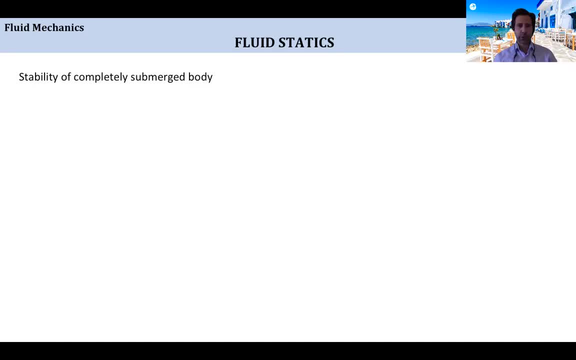 the displaced volume. and this location, which is the center rate of the displaced volume, is called the center of buoyancy, and we know that buoyancy force is vertical, acting through the center of buoyancy. okay, so now let's consider the stability of completely submerged objects first. 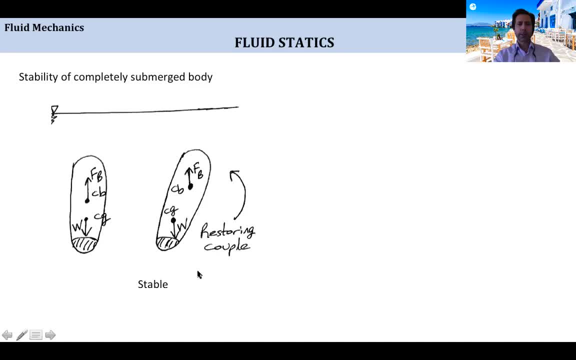 so first consider that we have such a submerged object. let's mark the bottom of the object so that we know that this is the bottom portion. this is the top portion. let's say, in the first case, center of gravity is located here for this object and center of buoyancy. 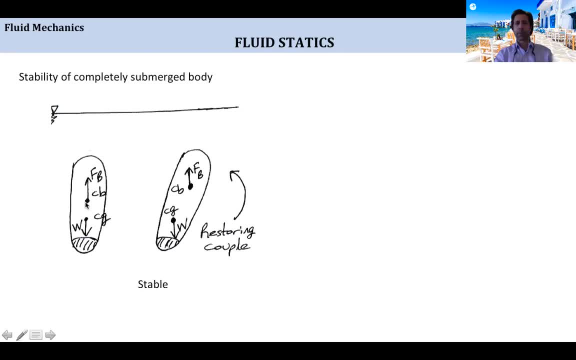 is somewhere here. okay, so we know that buoyancy force will be acting vertical up through the center of buoyancy, so as shown here, and weight will be acting downward through the center of gravity. now consider that somehow this object, this submerged object, is disturbed. for example, a wave passes over this. 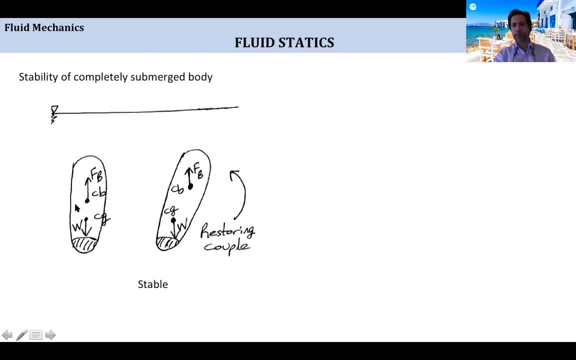 object. So there is a force that tries to flip this submerged object- Now let's say the object flipped as such- to the right. So our buoyancy force is still acting vertical and our center of buoyancy is located here. Our weight is still acting downward, as shown here through the center. 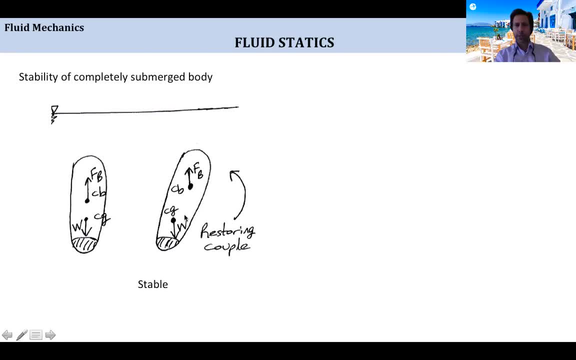 of gravity. So buoyancy force and the weight forms a couple that rotates, that has a direction in the counterclockwise direction. So buoyancy force and weight forms a restoring couple And this restoring couple, so basically this couple which tries to take the object back to, 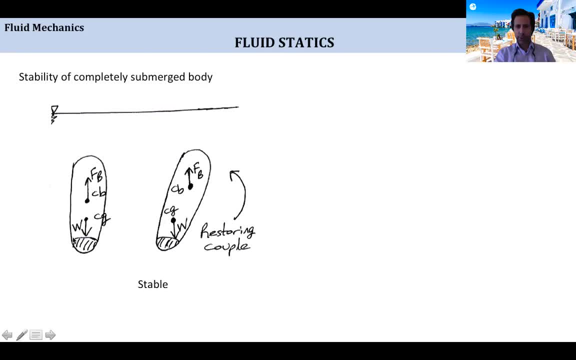 its original equilibrium position. So this was the starting position. It was disturbed and, because of the combination of the buoyancy force and weight, locations and directions, now a new couple formed which tried to restore back to its original position. So we can say that this configuration is a stable configuration. 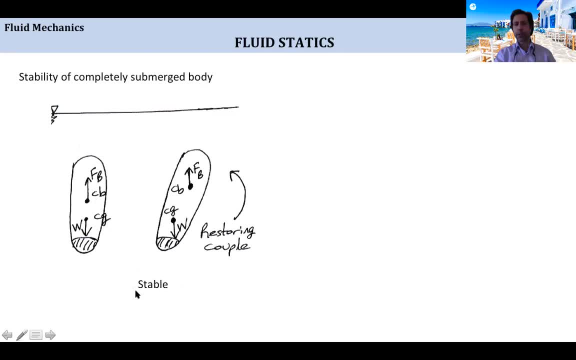 Okay. So when we have center of gravity is below center of buoyancy, we observed a stable configuration. So we can say that this configuration is a stable configuration. So we can say that this configuration is a stable configuration. Now let's consider another scenario. In this case, let's say we have center of buoyancy, that is, 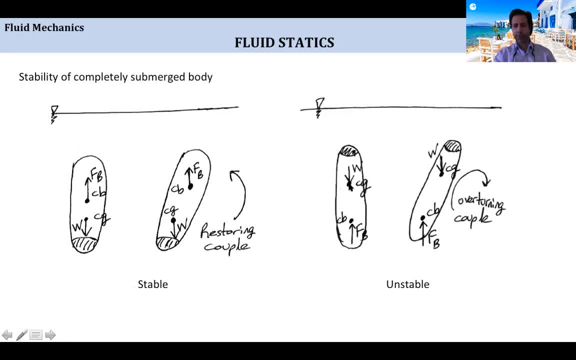 below the center of gravity here. Okay, So you can consider that the object is flipped. Okay, And let's say we have an equilibrium at this point, at this instant, We know that weight is acting downward through center of gravity. We know that the buoyancy force is still acting. 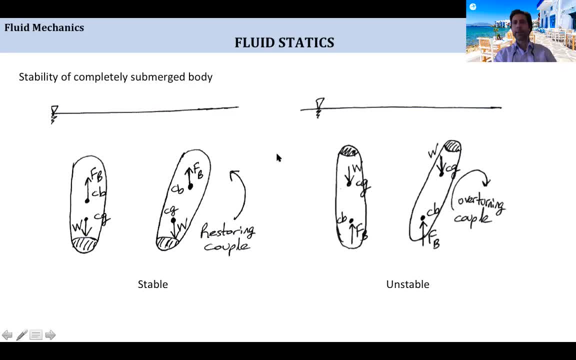 upward through center of buoyancy. And then again let's say we have a disturbance, let's say a wave hits on this surface and now the object is flipped as shown here. Again we have center of buoyancy. here buoyancy force vertical up. center of gravity: here weight is acting downward. here Now this: 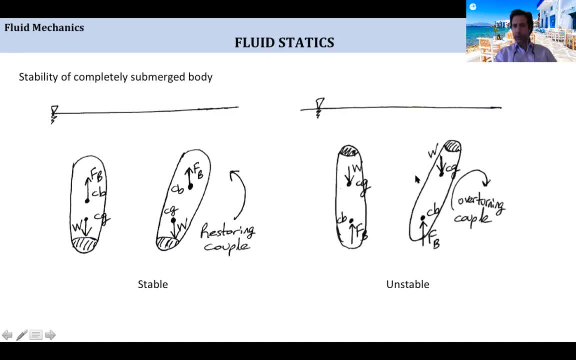 combination of weight and buoyancy force is acting downward. So we can say that the weight is acting downward here, And then again let's say we have center of buoyancy. here buoyancy force is acting. buoyancy force and their locations and directions will form a clockwise moment right. 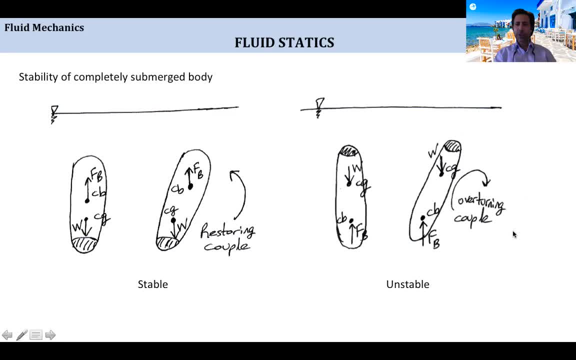 So we will have a clockwise moment which will try to overturn the object from this location. Basically, instead of trying to rotate the object back to its original position, now it's trying to rotate the object so that it deviates further away from the original. 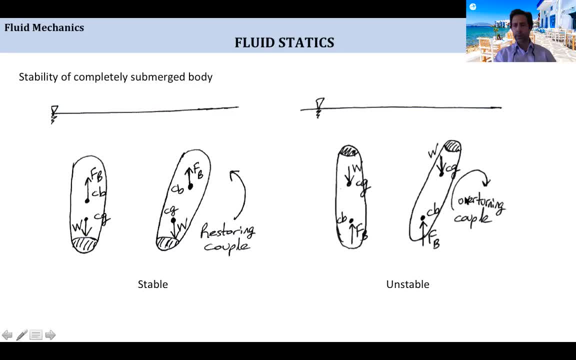 location. So we call this overturning couple, and this is because it is not going back to its original location. We call it an unstable configuration. So now, from this discussion, an important rule of thumb is that when the center of gravity is, 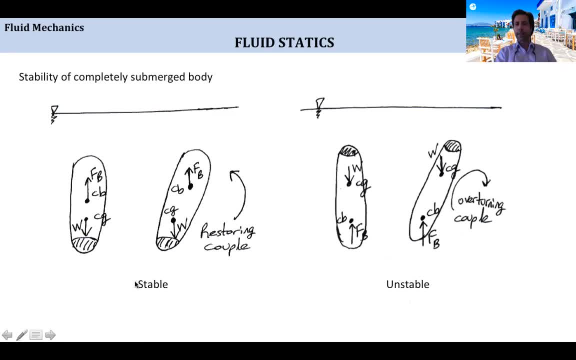 is below the center of buoyancy, we have a stable configuration. When we have a center of buoyancy that is below the center of gravity, we have an unstable configuration, and this is valid for all submerged objects. Now let's consider the stability of floating objects. 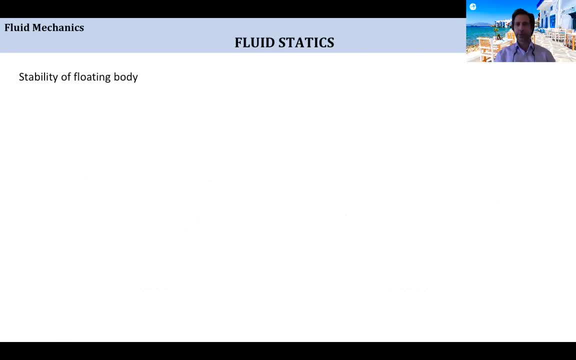 This is much more complicated than the stability of submerged objects. And let's see now why. First consider we have such a, let's say, object, okay, And we know that center of buoyancy is at the centroid of the displaced volume. 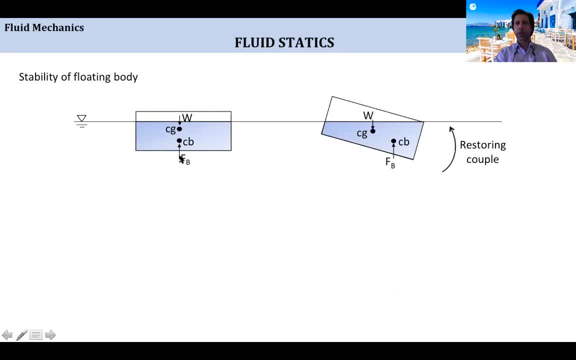 So let's say roughly, somewhere here, center of buoyancy. We know that buoyancy force acts through the center of buoyancy here. Center of gravity is somewhere here. Weight is vertical down at this center of gravity. Okay, Boise at this. you know, vertical weight is acting vertical down through the center of 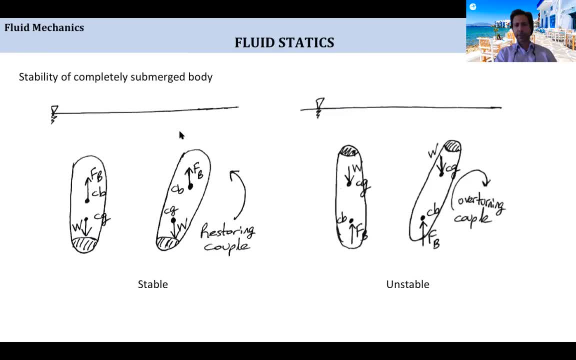 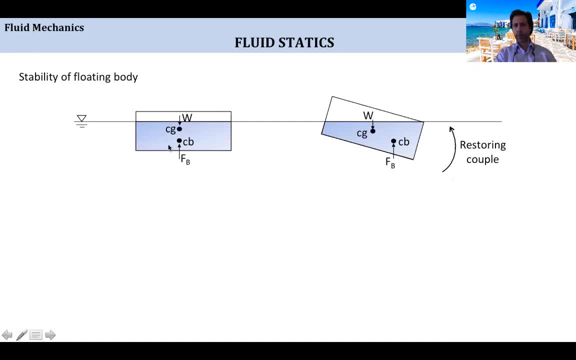 gravity. Now from the previous schematic, If you remember, center of buoyancy, below center of gravity, it should be an unstable location on stable configuration Right, But it's different for floating objects. Now let's say we have a wave. hit again on this. 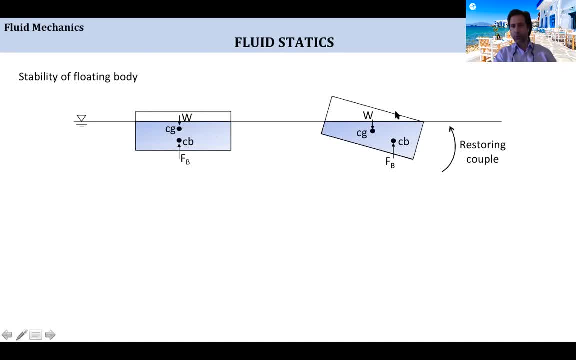 object. Now it is disturbed from the original equilibrium position and Our center of gravity remains the same. It is the same location. weight is still acting through the center of gravity. However, center of voice location changes because, by definition, center of buoyancy is at the center of the displaced volume. Now this place, volume changes. 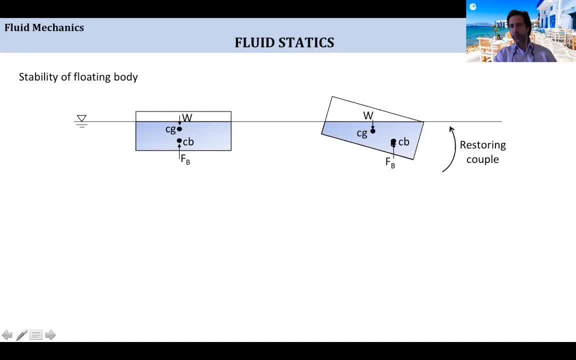 as you can see here, And so the centroid is, let's say, here. So center of buoyancy location is here, buoyancy force acting X vertical up. So this combination of weight and forces, buoyancy force, and Their action, location and directions will form a moment that tries to restore the original. 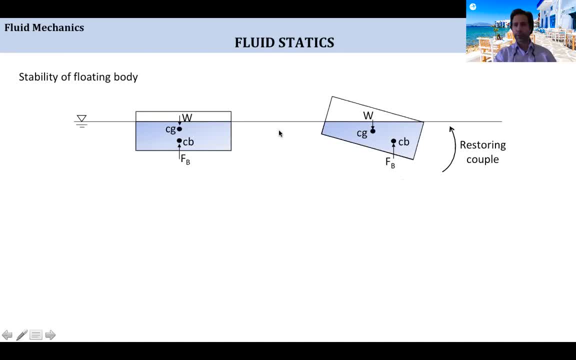 original position. original Position Position, Position of this: Unless a floating object- So we can say that this is a restoring couple- and object tries to go back to its original, Basically the position. Now let's consider a different case. Now our design is, let's say, a tall, relatively tall, slender object. Again, let's keep center of buoyancy below center of gravity. 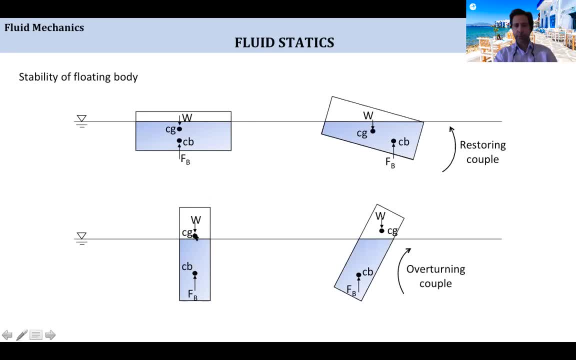 And we have buoyancy force acting up, great, acting down through the center of gravity. Now again this, This object, tall, slender object, is tilted due to some reason and we have Now: center of gravity location is the same, weight is acting downward. However, center of buoyancy location changes because the volume displaced changes and, as a result, we have: 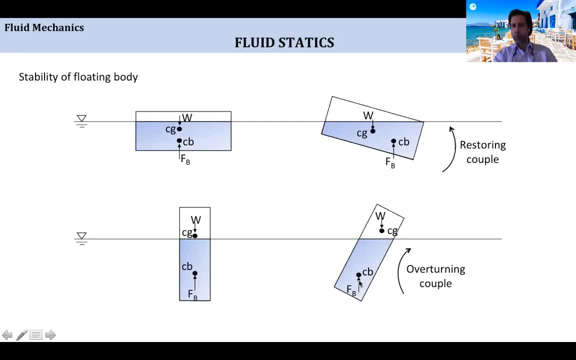 A new combination of buoyancy force and weight and their action location and directions. So you can see from the schematic that the moment forms through this combination of forces and their Action locations is in the clockwise direction. So this Configuration leads to further deviation from their 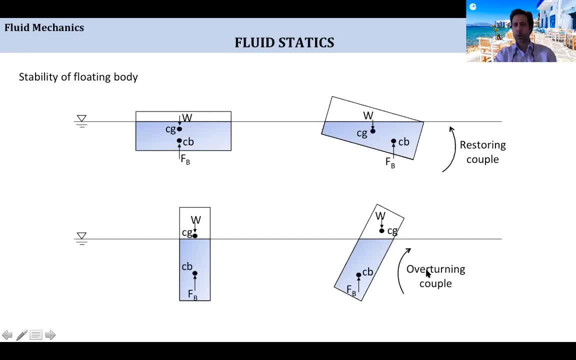 original equilibrium position. so this is an overturning couple. so while the first- the top configuration- is a stable configuration, the bottom configuration, you can see- the second, the tall, slender object, has an unstable configuration and yet both have the center of buoyancy below center of gravity. so this means that we cannot come up with a generalized. 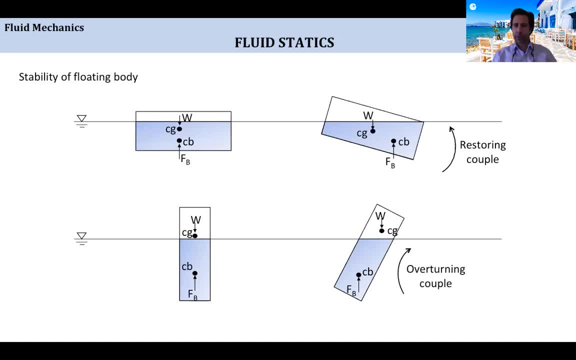 rules for stability of floating objects. we could come up with a generalized rule for stability of submerged objects, as you have seen in the previous slide. so, which means that when we have a floating object, we need to do a detailed analysis, and this is the case for the ships right.